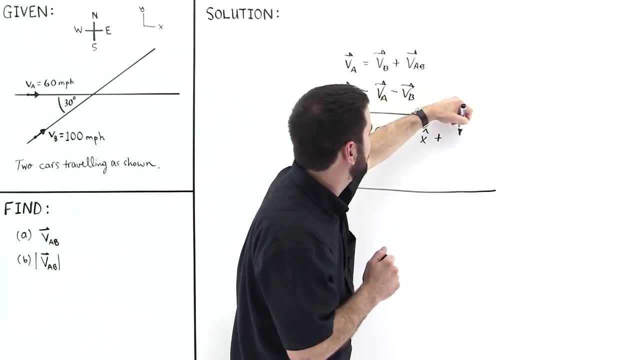 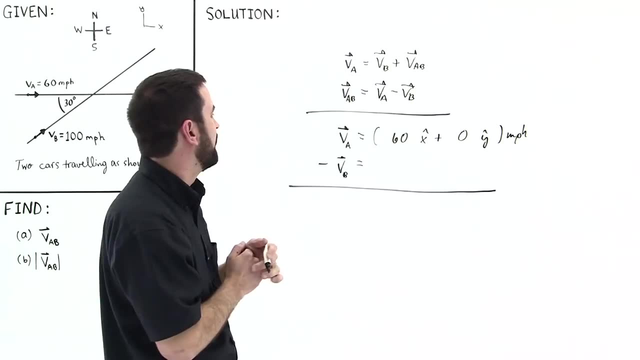 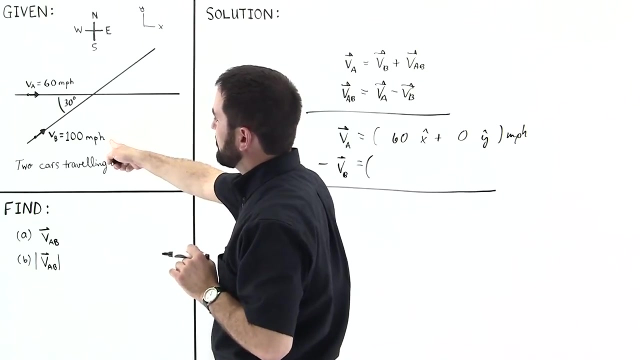 And then, as usual, we annotate that this does not have a Y component, right, Like so, And we'll see how that works, because then we can just this minus this to give the resultant component here. Okay, then this: the velocity for B does have components, right. 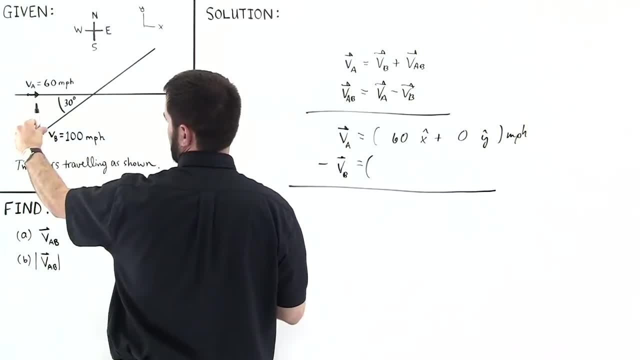 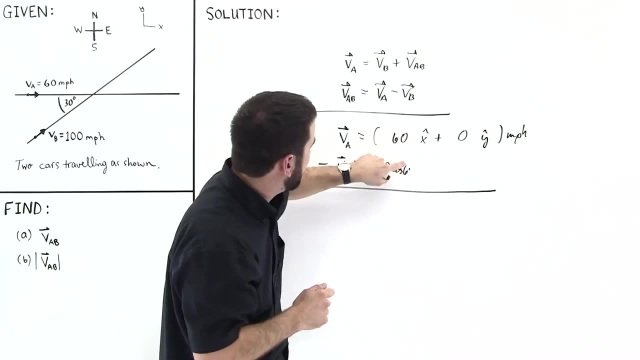 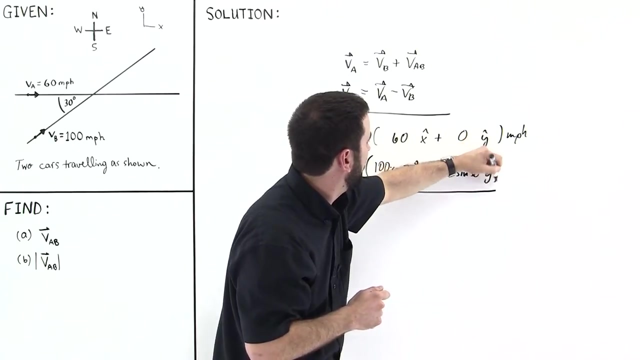 It has an X component, a positive X component and a positive Y component. So we have 100 times the cosine of 30.. X hat plus 100 times the sine of 30 degrees. Y hat minus power, right. 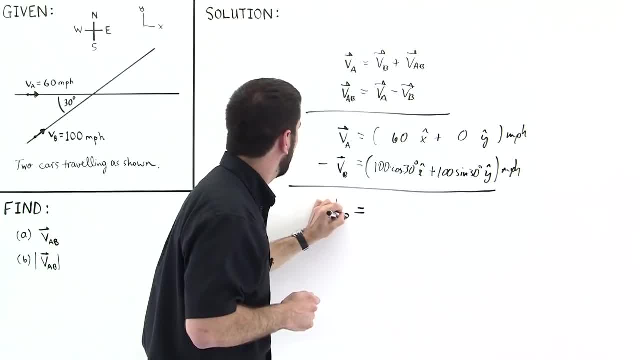 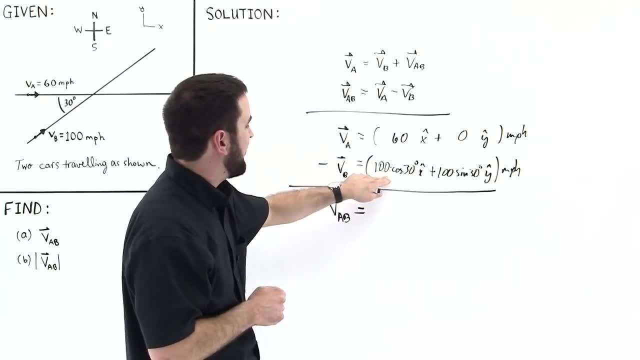 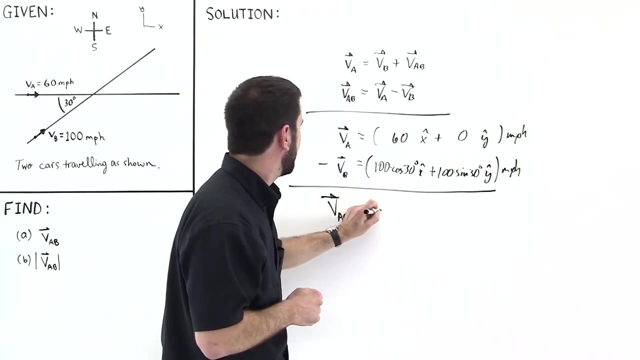 Okay, so then the velocity of A relative to B will be equal to this minus this. This is 86.6, so 60 minus 86.6 is negative, Negative 26.6, so negative 26.6 X hat. 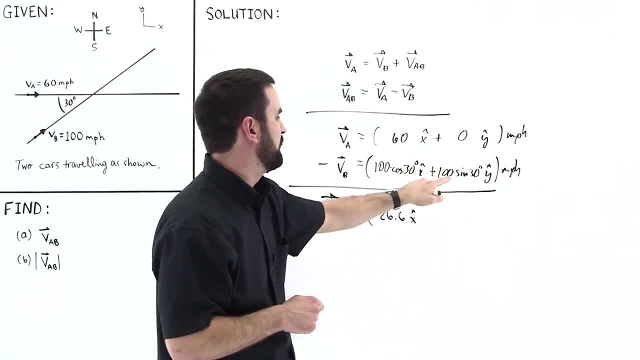 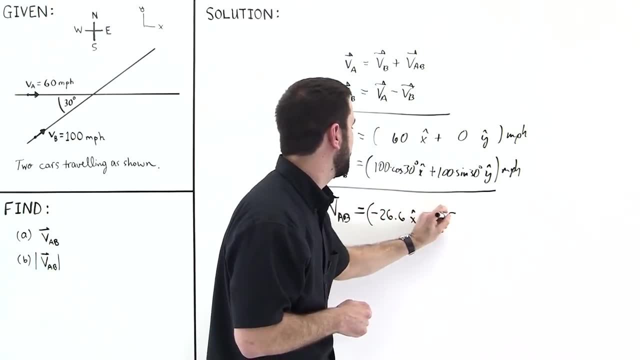 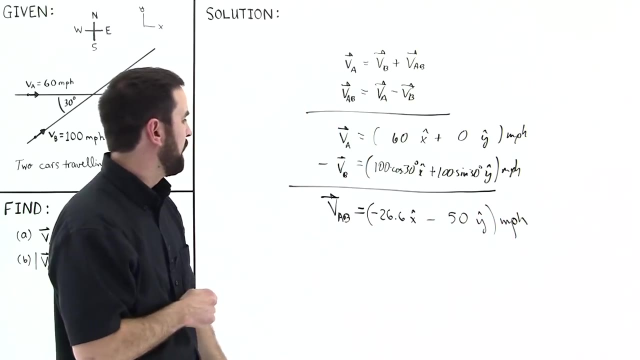 And then 0 minus this, this is sine of 30 is a half, so this whole thing is 50.. So this is minus 50 Y hat, and that's in miles per hour. right, Okay, so this is part A. 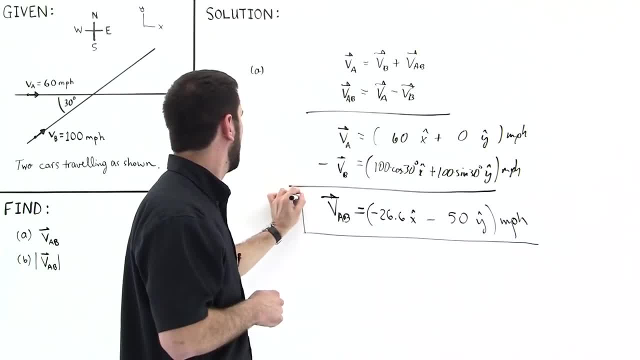 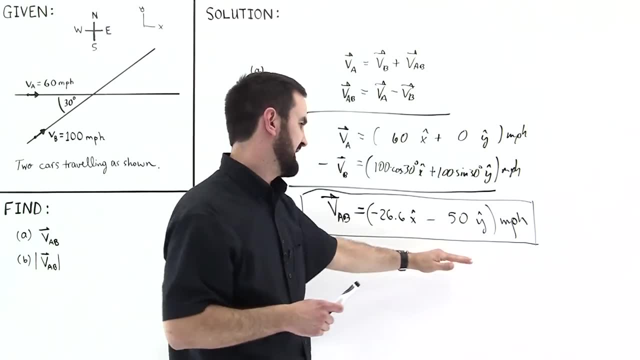 Let's take a look at what this vector is. It's telling us. it says: first of all, let's take a look at the Y component first. It says that the Y component is negative, 50 Y hat. And that makes sense because this guy is traveling towards this guy. 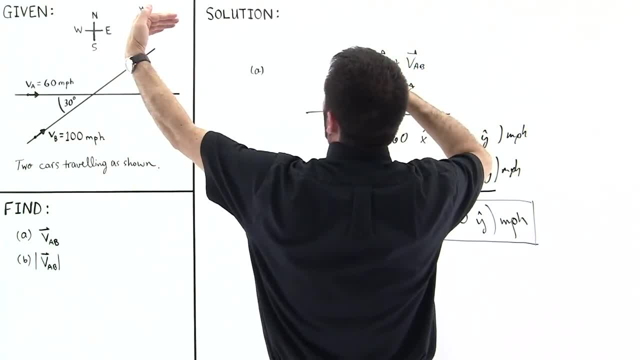 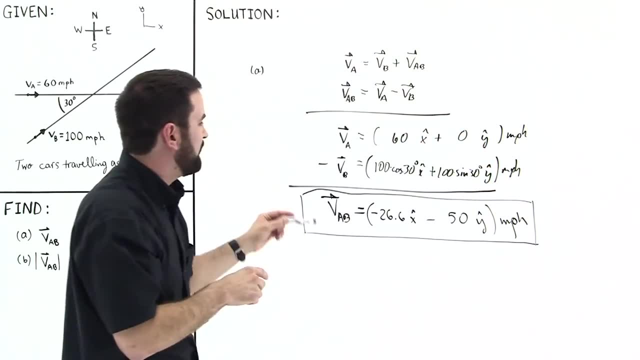 So if we're sitting in this car, we're seeing this guy, this guy over here, we're seeing him come closer to us, right, But we're also traveling 100 times the cosine of 30.. Cosine of 30.. 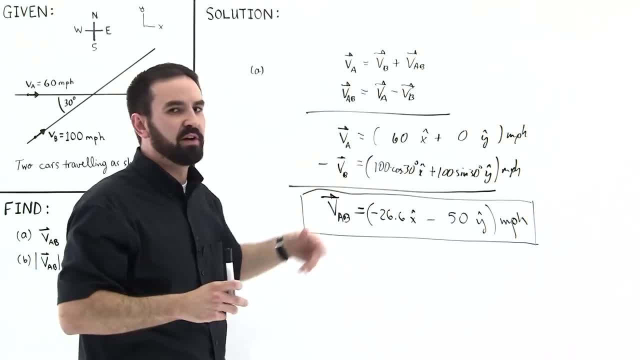 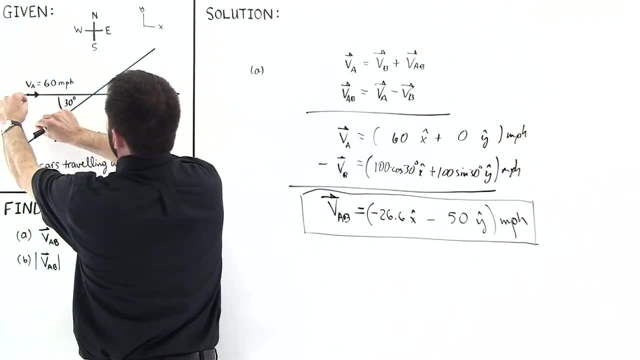 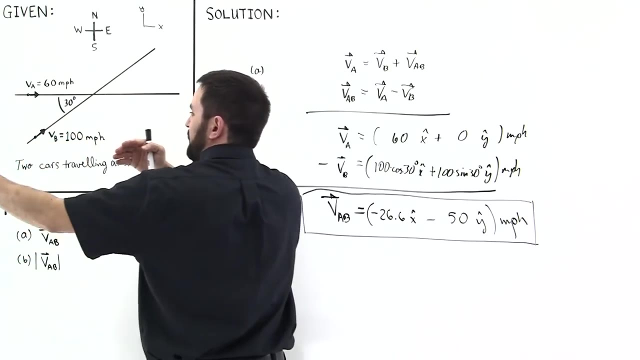 Cosine of 30 is 86, cosine of 30 is 0.866 times 100 is 86.6.. So we have a faster velocity in the X direction. So we're actually traveling faster than him like this. So we actually see him, we see ourselves, we see this guy moving away from us.